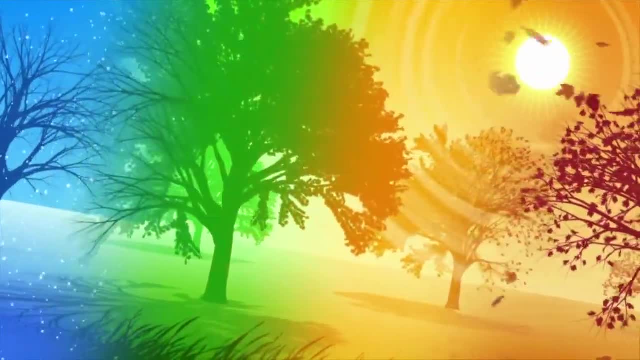 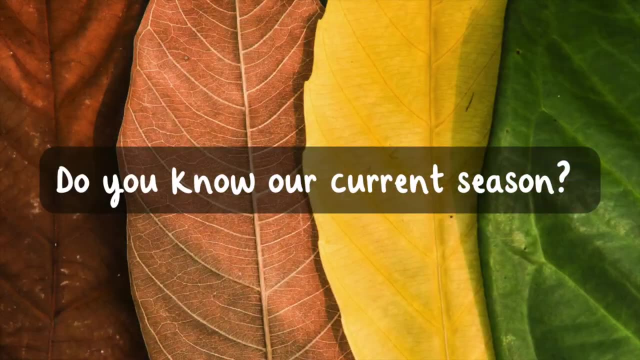 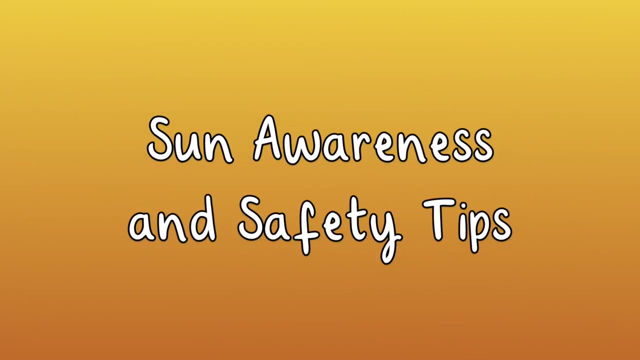 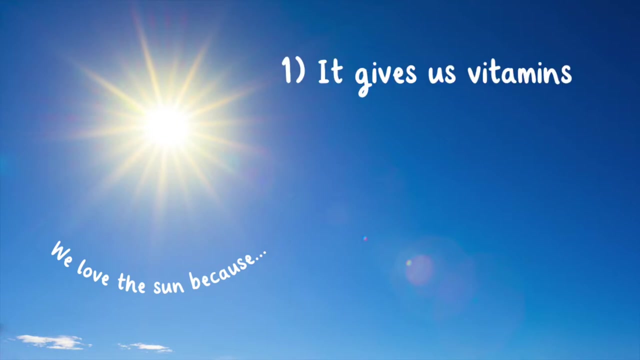 Many parts of the world have four seasons in a year. They are spring, summer, fall and winter. Do you know our current season, Summer? Sun awareness and safety tips. We love the sun because it gives us vitamins. it's healthy for our bodies and our minds to play and learn outside the sun. 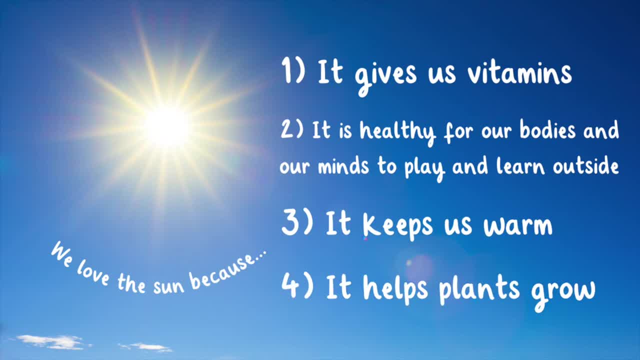 keeps us warm and the sun helps plants grow. But we have to be careful in the sun because it can hurt your skin by burning it. Have you ever been sunburned? Give a thumbs up if you have been sunburned. Give a thumbs down if you've. 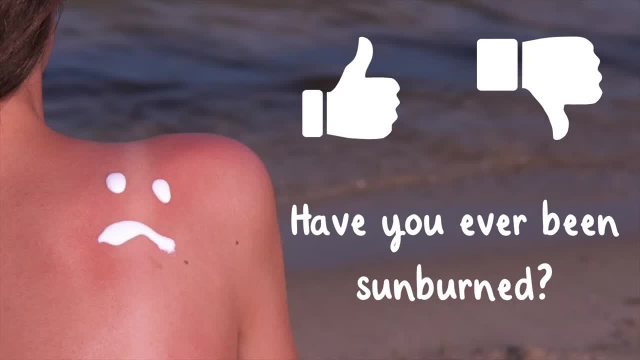 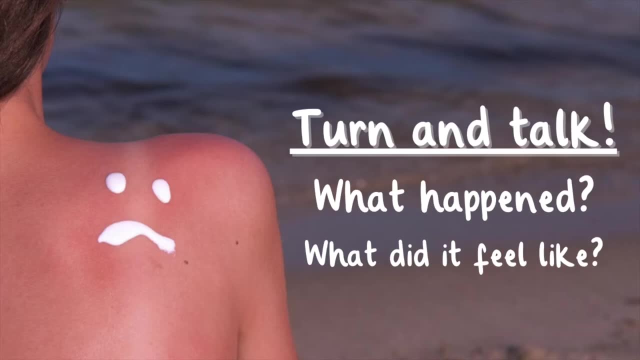 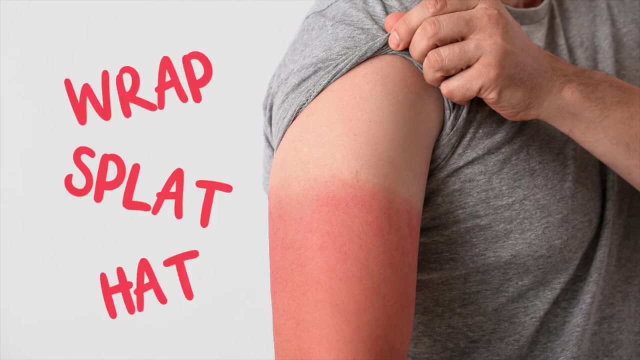 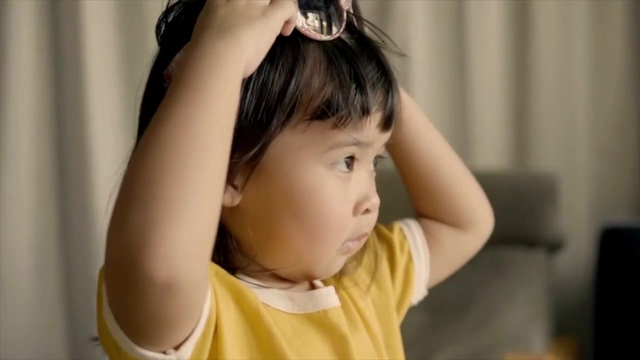 never been sunburned. Turn and talk. What happened? What did the sunburn feel like Here at Twinkle? we like to use the wrap splat and hat method: Wrap, Wear sunglasses to protect your eyes, Cover yourلا. 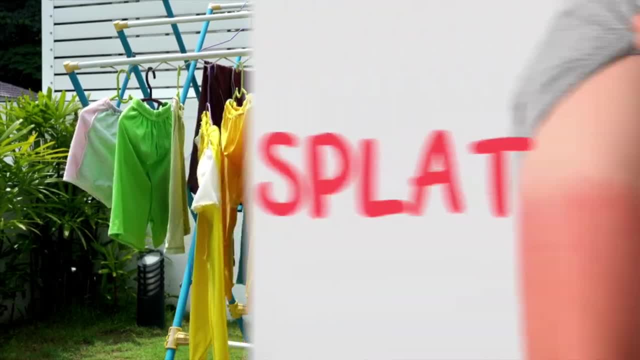 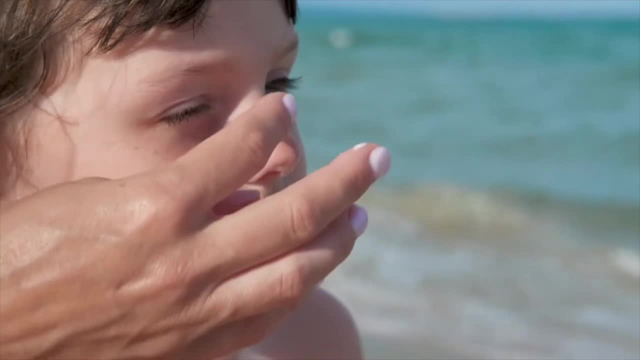 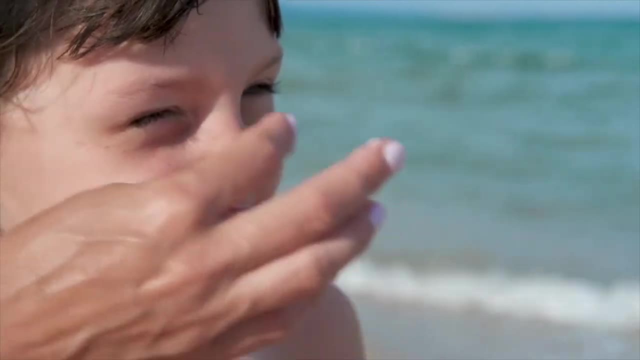 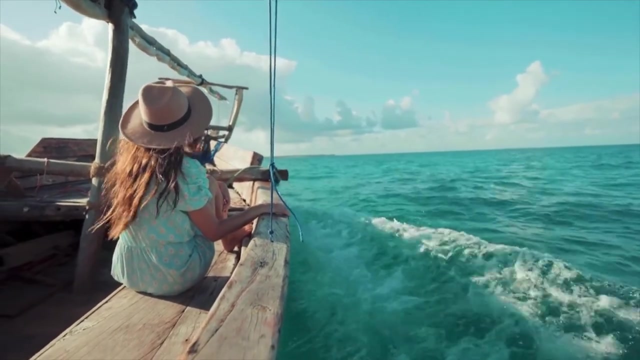 bodies with t-shirts and shorts. splat: use sunscreen to protect your skin. we recommend to wear sunscreen on any parts of skin that are not covered, including your face, nose, ears, neck, arms and legs. hat: wear some hat to shade your face and neck. we recommend wearing a wide brimmed hat to keep your face and neck shaded. 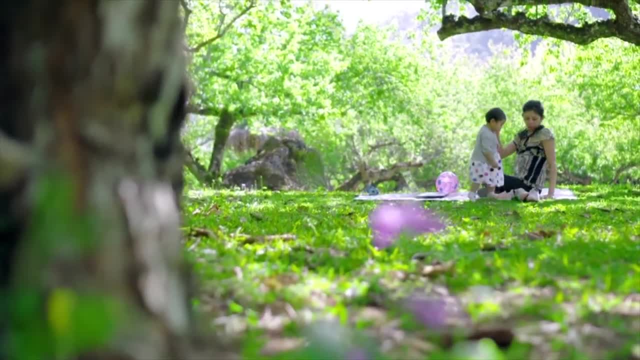 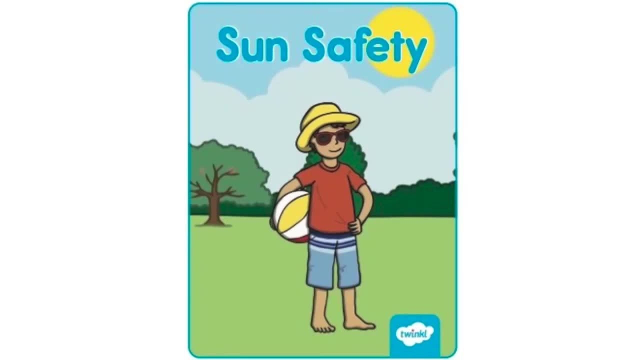 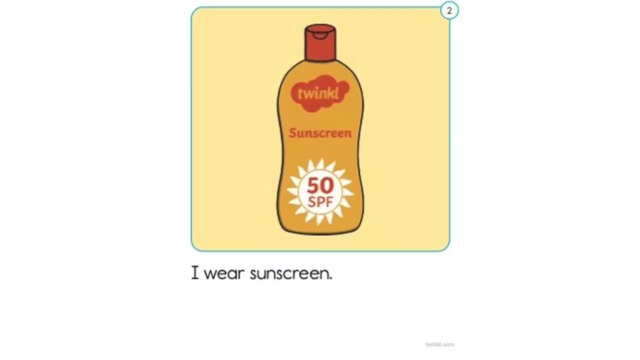 last but not least, play in the shade and drink water to stay hydrated. sign safety: I know how to stay safe in the Sun. I wear sunscreen. I wear sunglasses. I wear glasses. I wear a sun hat. I wear a t-shirt. I play in the shade.